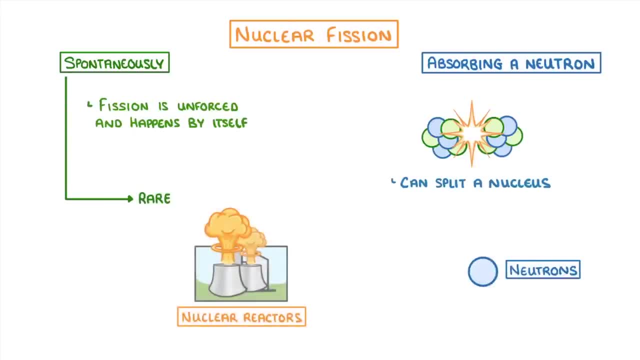 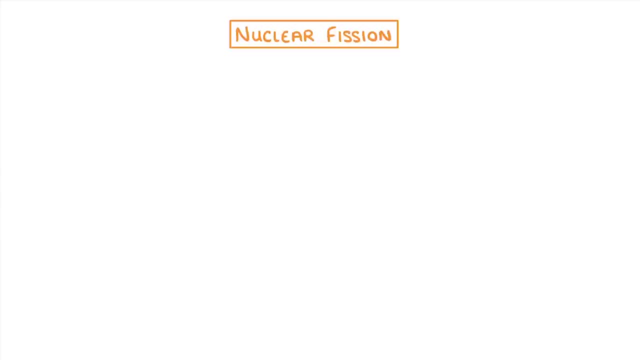 and so when we use fission in nuclear reactors, we have to use neutrons to get the process started. To understand how the process works, let's go through the steps. As we said, we start off with a large unstable nuclei like uranium-235, and we fire a relatively 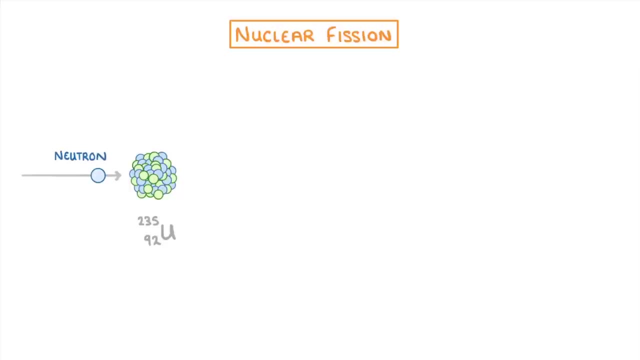 slow-moving neutron at it. This addition of a neutron to the nucleus makes it even less stable and causes it to split apart into two smaller nuclei that we call daughter nuclei. It also releases two smaller nuclei. Each of the neutrons can then go on to repeat the process all over again with another uranium. 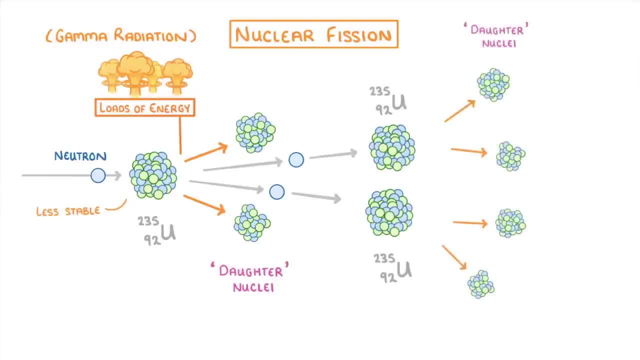 nuclei, and so more daughter nuclei energy and neutrons will be released, which again allows the process to start over Now. the key point of this process is that nuclear fission leads to a reaction to the nuclear fission. It leads to a chain reaction where the first fission can trigger more fission, which can 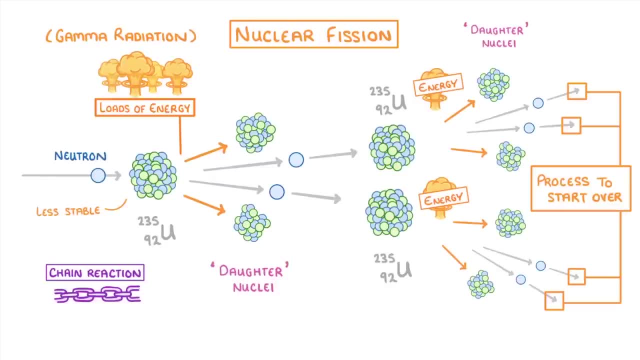 in turn, trigger even more fission, and so on. If this process isn't controlled properly, then the whole system can quickly get out of control and release huge amounts of energy, which is exactly what happens in a nuclear bomb. In nuclear reactors, though, the rate of fission has to be carefully controlled. 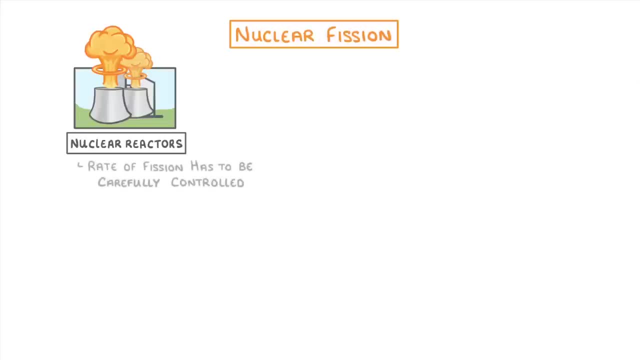 This is mainly achieved by control rods, which can be lowered into the reactor to absorb the neutrons and so slow down the reaction. Meanwhile, the energy released from the process is used to heat up water and turn it into steam, which can then drive turbines that are connected to an electricity generator. 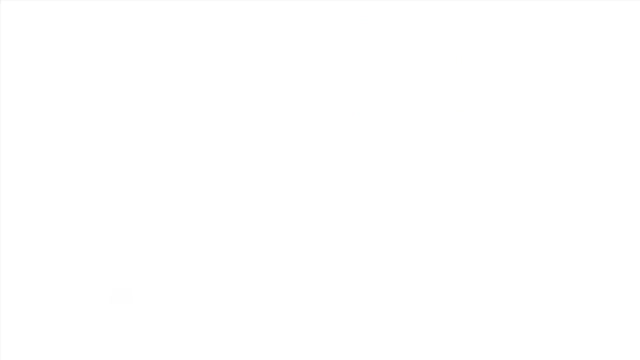 The last thing we need to cover are the pros and cons of nuclear energy. The pros are that the uranium or plutonium fuel is relatively cheap and it produces a large and steady amount of energy. And although it's not classed as a renewable energy, it is clean as it doesn't produce.